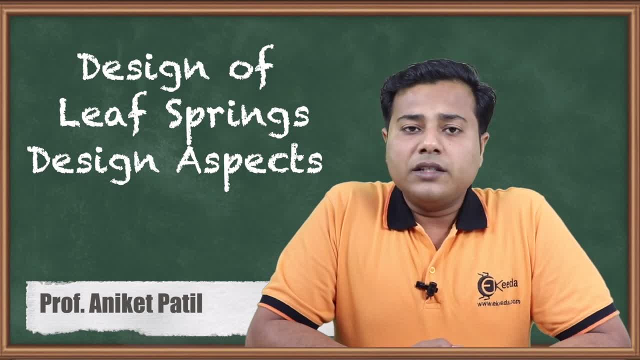 In today's session we are going to start with a new part of this lesson, which is nothing but lift design or lift spring design. In the previous to previous session, we have already seen different terminologies associated with lift spring and its significance. Let's quickly revise: what are the significances, what are the terminologies and what is the design procedure? 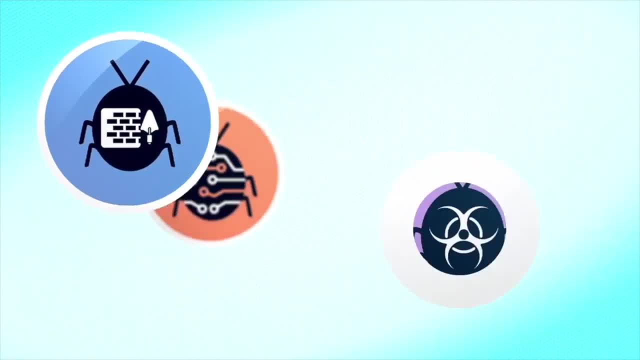 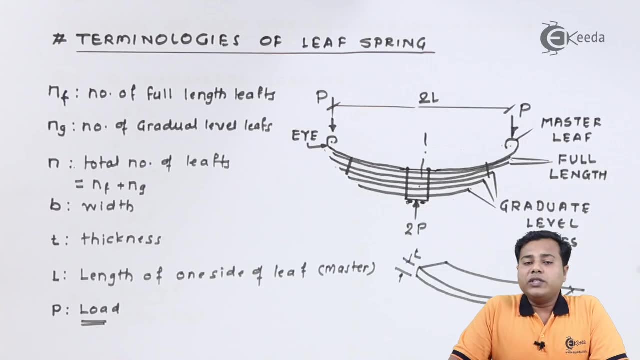 So let's begin. So, students, you can see on the screen different terminologies and the schematic associated with this lift spring given. If you see this properly, this is how the structure of lift spring is explained, where different plates of this particular schematic are used. 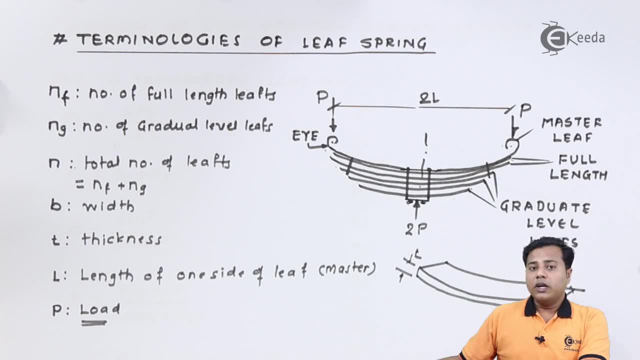 Where this particular thing or this particular dimension is called width of the lift spring. This is the thickness and of course these are the different lengths And if you see, there is a curvature. So there is always some radius associated with the lift spring. 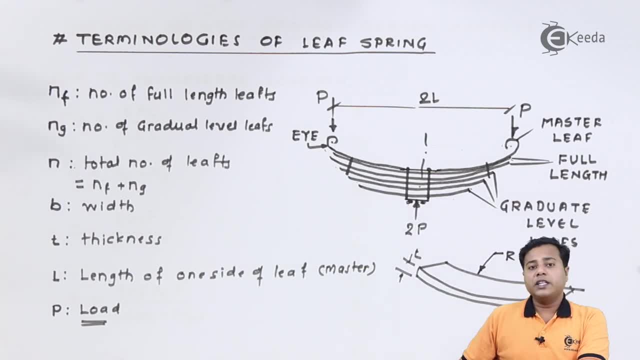 If you see, lift springs are made up of different plates of certain thickness and certain width, Of which there are different sections, which you can see, and there are different divisions for them. For example, if you see, the length of the springs or the lifts are going to change or are changing gradually. 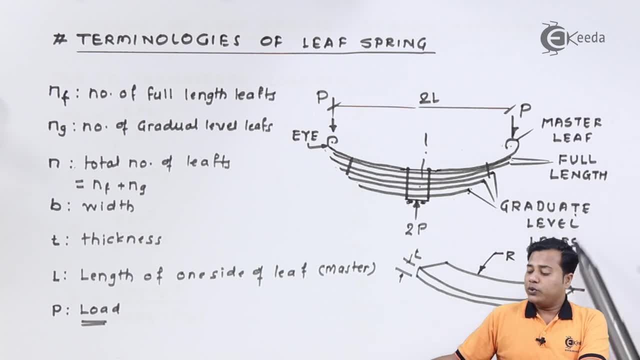 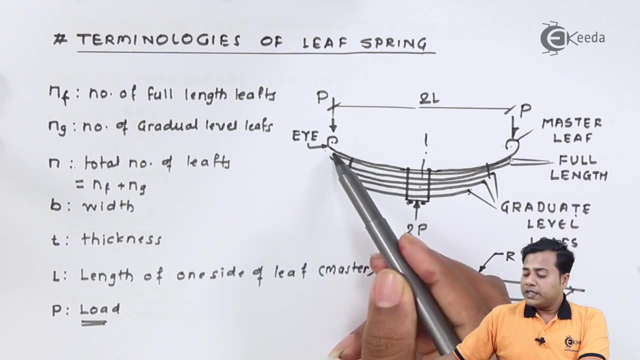 And that's why they are called graduate level lifts or graduated lifts. The number can vary from 3 to 12.. Also, but it depends upon the given application. Further, if you see two lift springs or two lifts of that particular spring, they appear to be of same length and they are called full length springs. 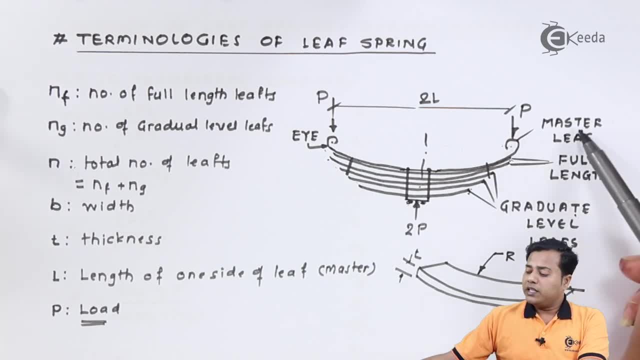 They may be two or three numbers, And last one is the master lift. Master lift is the longest one and it has the ends bent so as to form the eyes. These are called the eyes of the lift spring. Now, when these eyes come into picture, the eyes are actually. 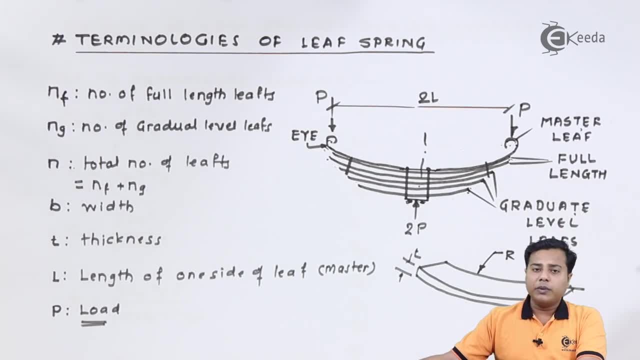 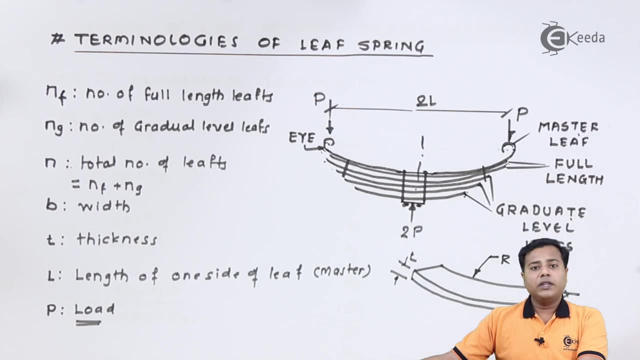 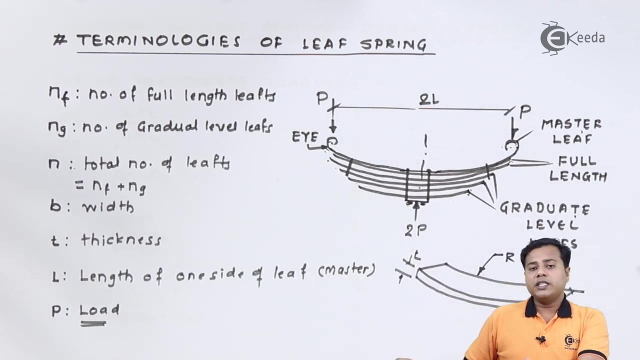 Bolted together with the application, for example, vehicle, automobile, where these lift springs are used. So the body of a vehicle will be bolted with this particular eye, with the given lift spring. Further, if you see, the total force acting on that particular one lift spring is divided, or it is assumed to be divided, into two sections. 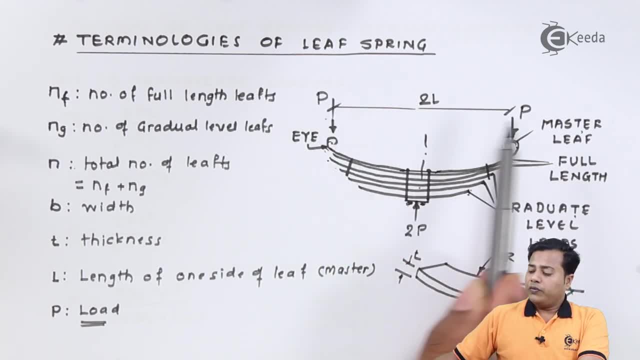 So the load is 100 Newton or 100 kilo Newton. 50 kilo Newton on either side will be applied accordingly. Next is the center Center distance. as far as the master lift spring is concerned, It is assumed that 12 is the length. 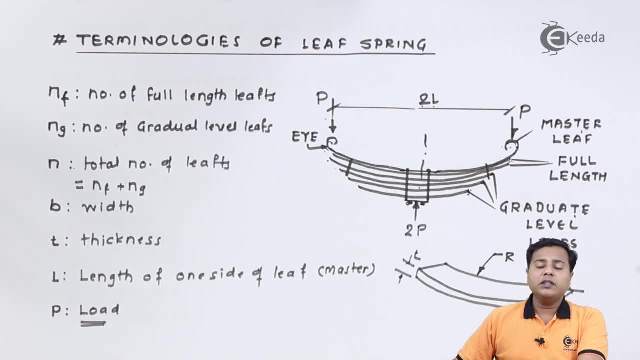 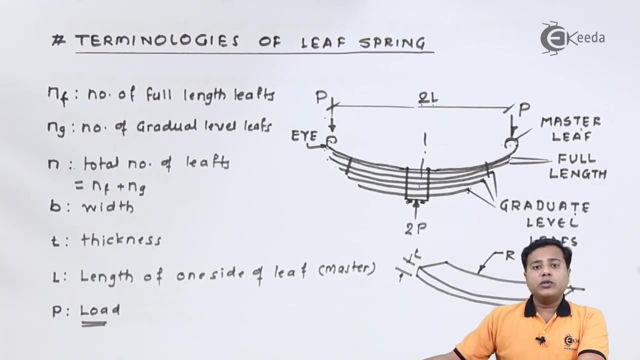 So accordingly, the parameter will change: if length is 100 millimeter, the center to center distance will become 200 millimeter, and so on. So these are the important terminologies. Now, of course, there are many assumptions which are made in the analysis of this spring. 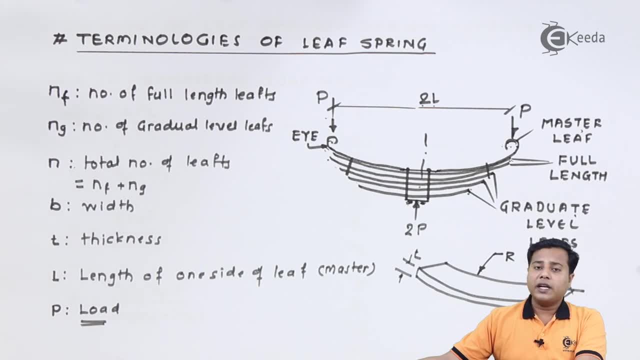 But since the syllabus is restricted to the design aspect and the applied design aspect, we are not going into the depth of the derivation part. Let me just tell you That the complete structure of flip spring, If you look at the force applied, it carries the transverse loads and hence for transverse loads, 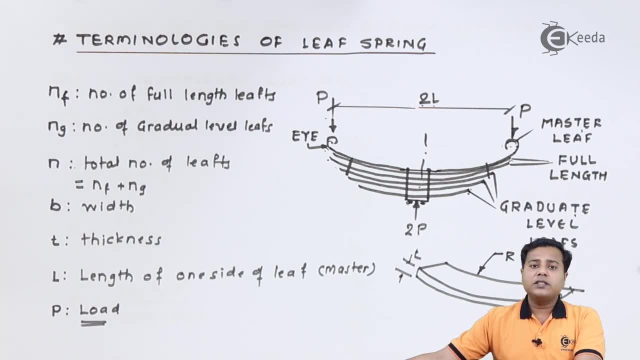 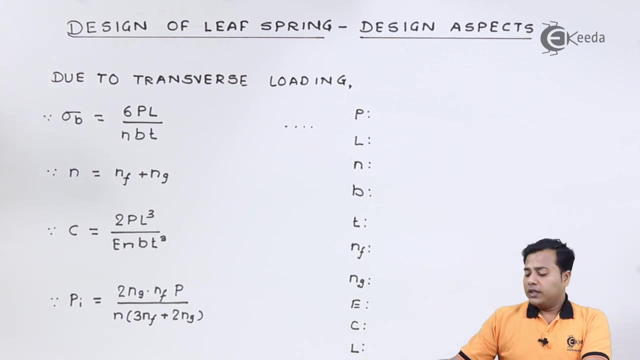 Whatever these traces come into picture- maybe bending stresses, shear stresses or any other normal stress- are considered together for this particular derivation And based on that, certain formulas are made up which we are going to look at in today's session. So there are few formulae which we have segregated based on the given course. 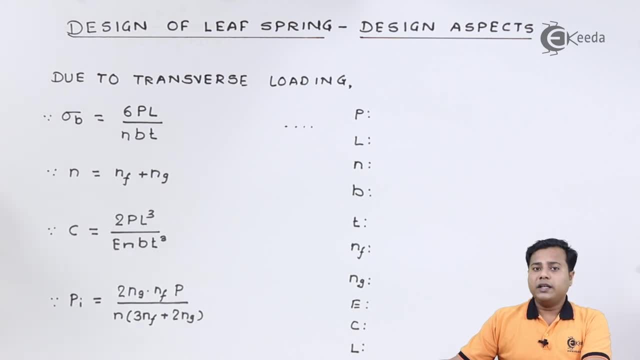 Of course, you can find all this formulae in the book of design data. So these are the four formulae which we are going to use for this particular numerical and, accordingly, the terminologies are mentioned. This is the bending stress based on the load acting, the length, the number of lips. 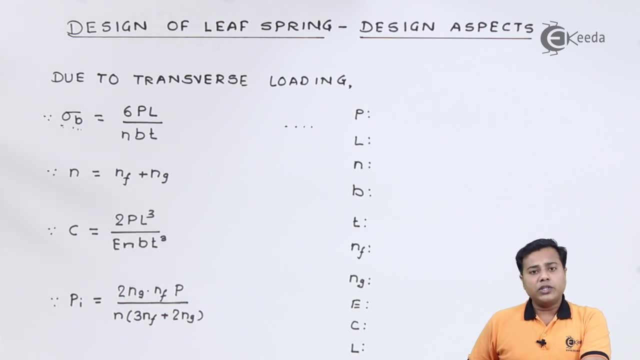 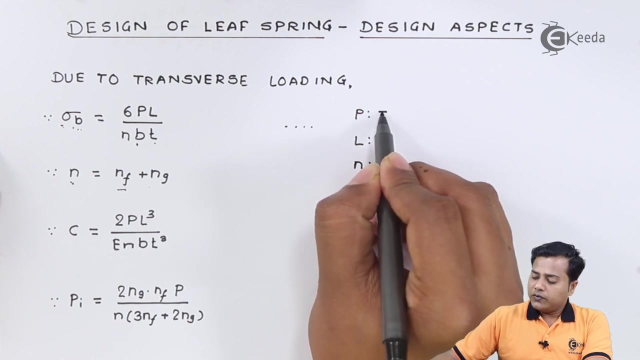 The total number of lips is, of course, the addition of graduated number of lips, the master lift and the full length lift. So in that case the full length lift plus graduated level lips numbers are collected to find the total number of lips. Then it is the width, and this is the thickness of any one lift and hence it's the transverse load. 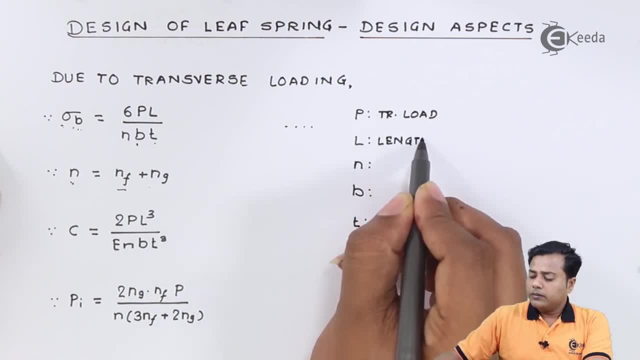 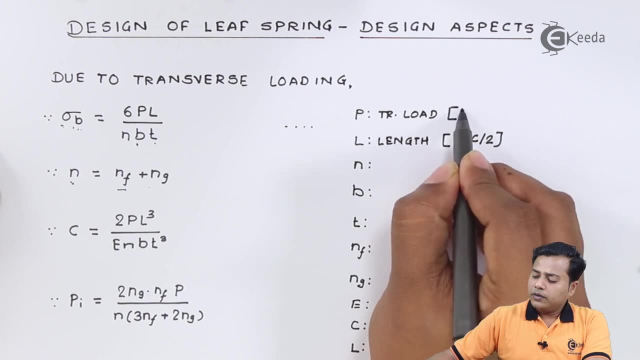 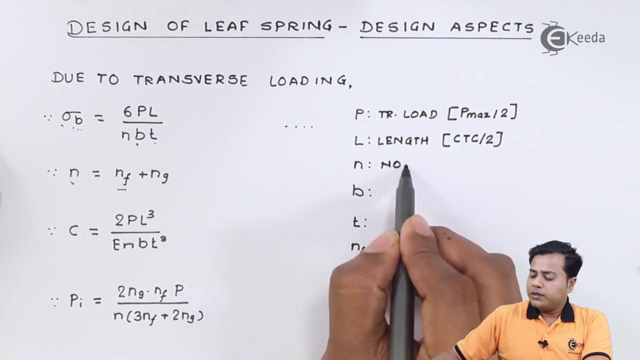 The length. Let's write it center to center. distance divided by two. This is P maximum divided by two and is the number of flips. Then it's the width of a lip, Is the thickness Of lips. This is the full length. 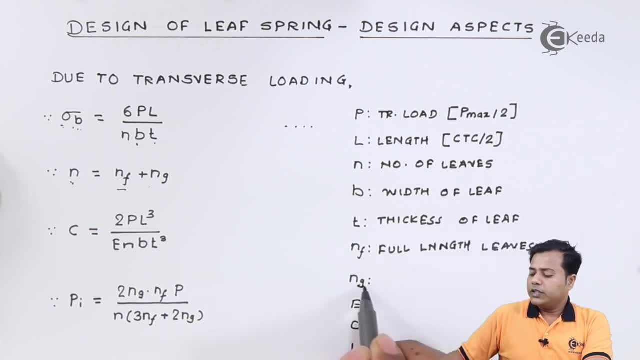 Lift or leaves number. This is the graduated lives, This is the coefficient of elasticity, or Young's modulus C. as usual, is a relationship. and last is the length, which is already mentioned. So n is the total number of flips. Further, the index is specified using this empirical relation. Let me repeat that the course does. 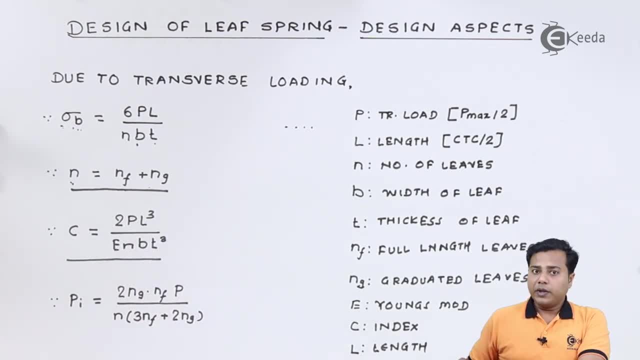 not enter in the derivation part. So we are going to apply directly- and you can find this formula in the book of design- and this is the pre stress which is required to make the spring initially at D, Given equilibrium. Now, this is an interesting topic We should discuss. on the structure, 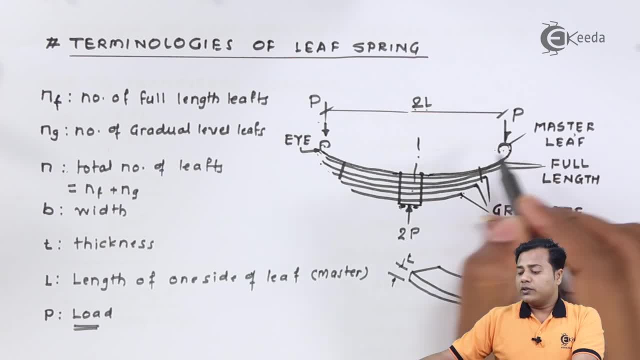 says that they are curved in nature. Basically, the transverse load is going to act on them Somehow. if you see, each and every spring which is graduated has different radius of curvature. in short, since they don't have the equal radius of curvature, They will have always some nipping. 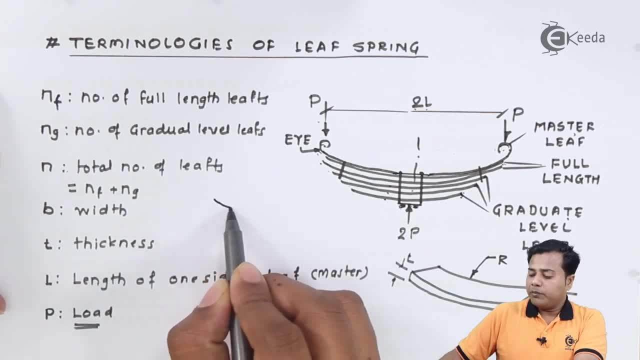 point in between them. So nipping point is nothing. but, for example, this is the 11th spring And let us say this is the 12th spring. In that case, there is always some gap that remains between them, just because the radial differences are there, and hence, in order to 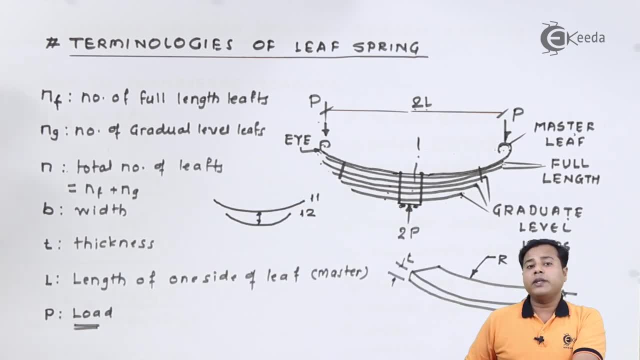 make them one body. they are initially traced by means of certain application, So they will be hold. they will be held together by means of certain load and certain bolts and due to this water action takes place. that is quite nipping of live. for this We require.